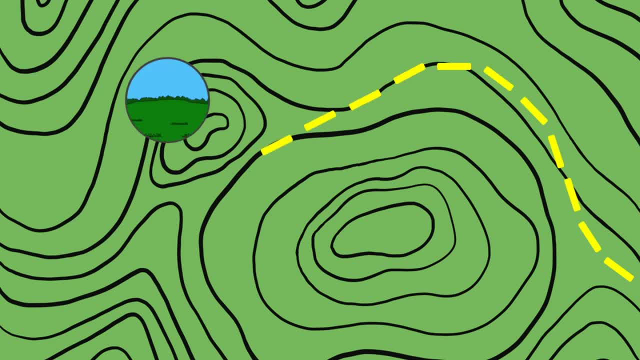 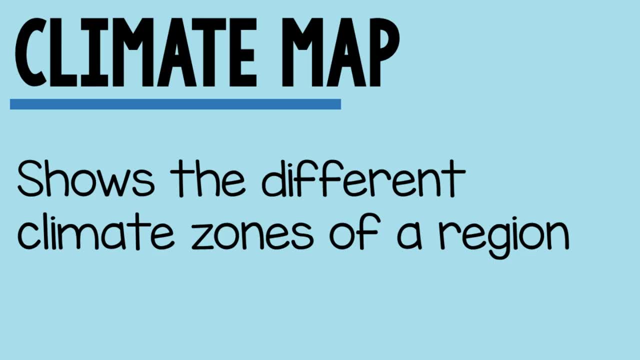 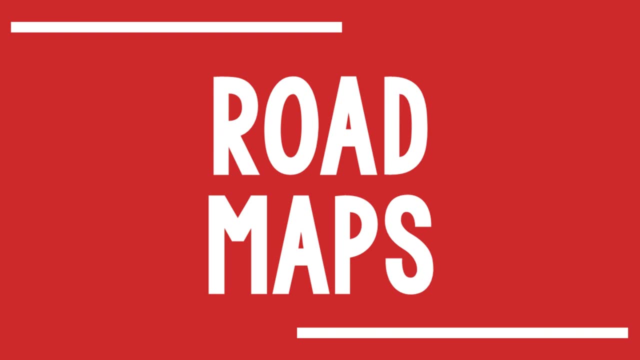 maps to navigate around different types of landforms like hills, mountains and valleys. A climate map shows the different climate zones of a region and provides information about temperature, precipitation and other weather patterns. Before you jump into your car and hit the road, you may plan your journey using a. 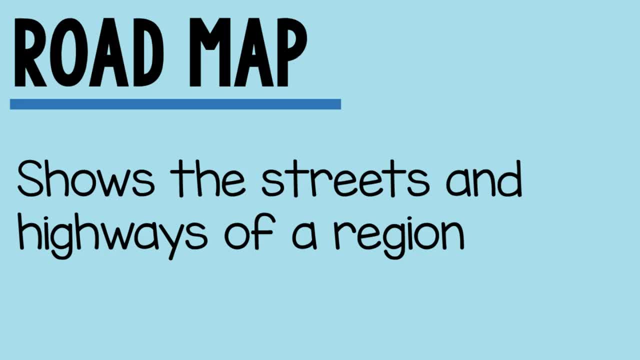 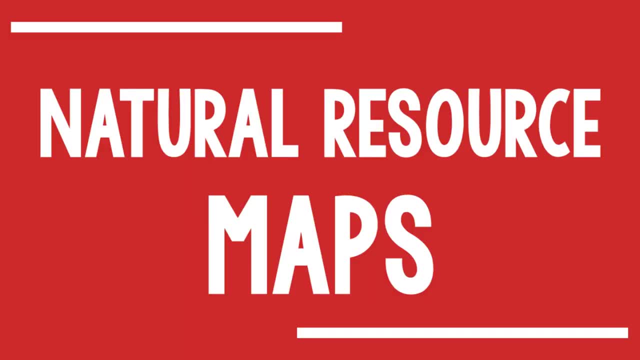 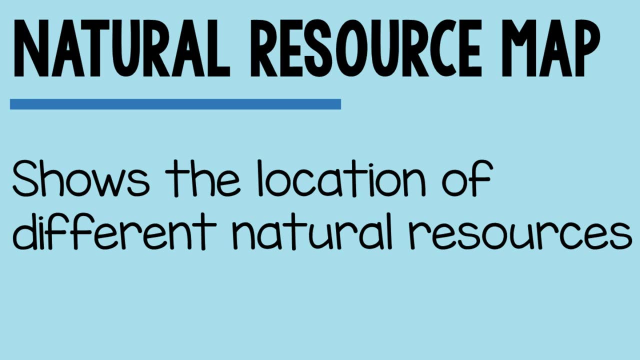 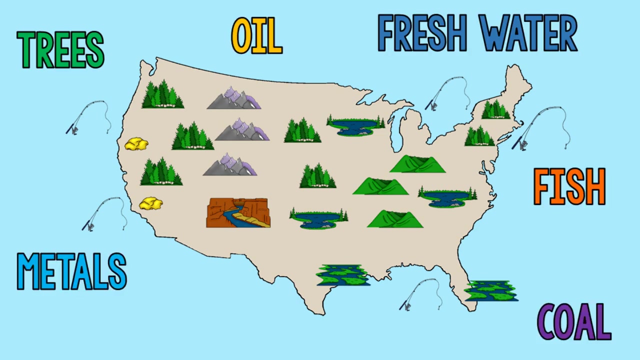 normal map. A road map shows the streets and highways of region. It can help us to navigate through unfamiliar areas and reach our final destination. A resource map shows us the location of different natural resources. Summary Examples of natural resources include trees, fresh water, fish, oil, coal, precious metals. 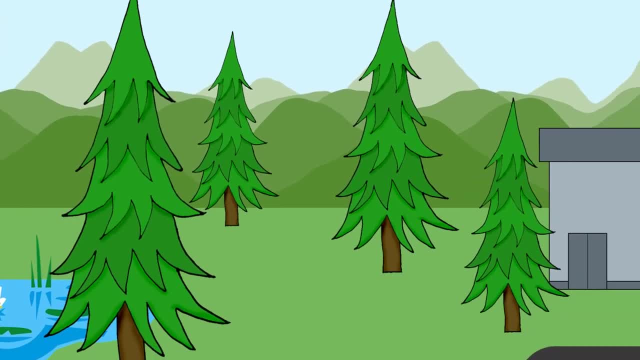 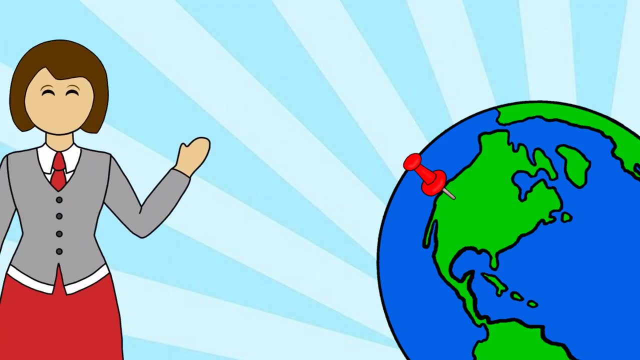 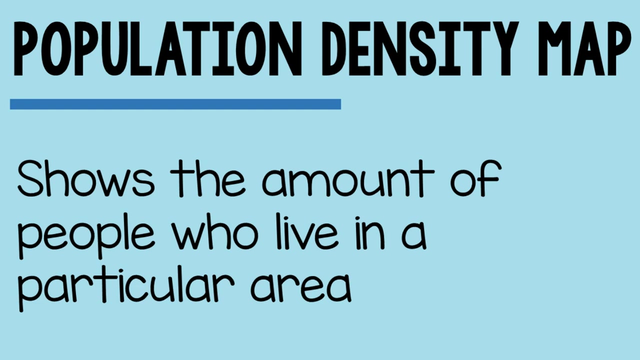 minerals and so much more. These resources are used by humans to make different types of goods. Have you ever wondered where people live around the world? A population density map can show you the amount or density of people who live in a particular area. 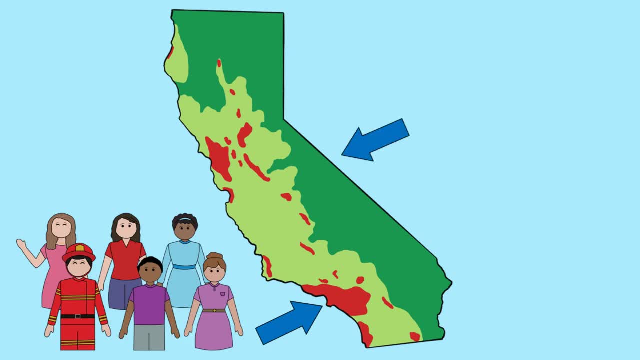 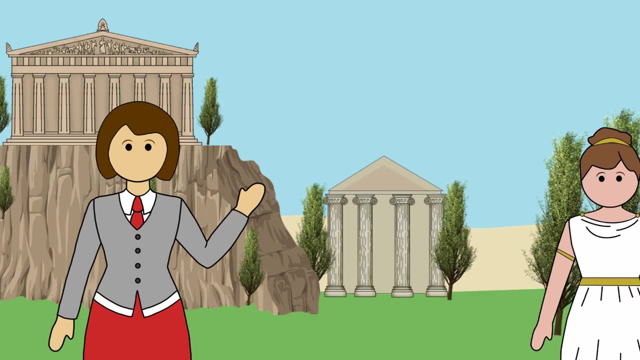 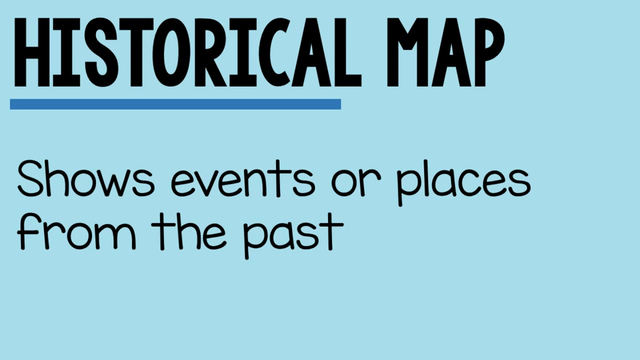 A city filled with people will have a higher population density than a rural area filled with farmland, where people live farther apart. When learning about the past, you may study a historical map. Historical maps show events or places from long ago, like battles, the locations of ancient 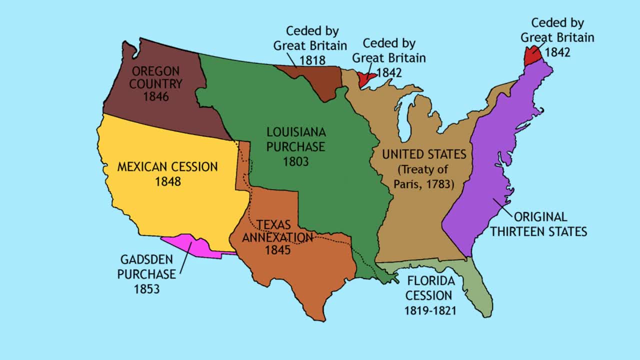 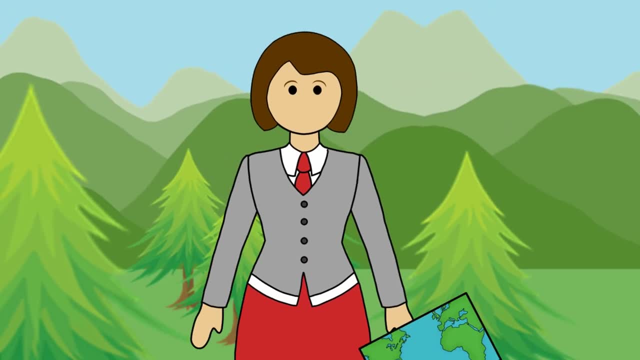 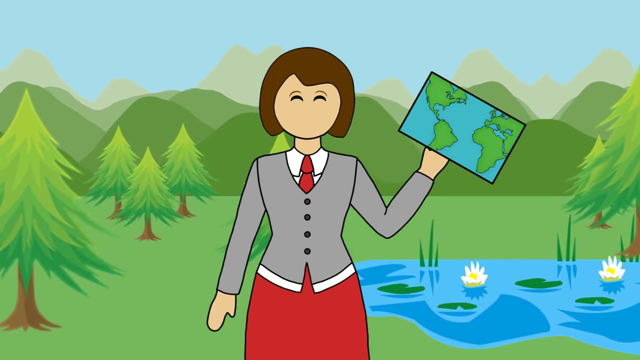 civilizations, borders that have changed over time, and more. Okay, I think I figured out which map to use. There are so many more examples of different types of maps. Each serves a unique purpose And can help us understand the world around us, no matter where we find ourselves. 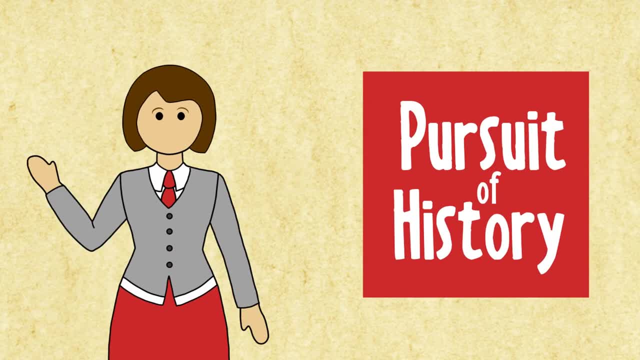 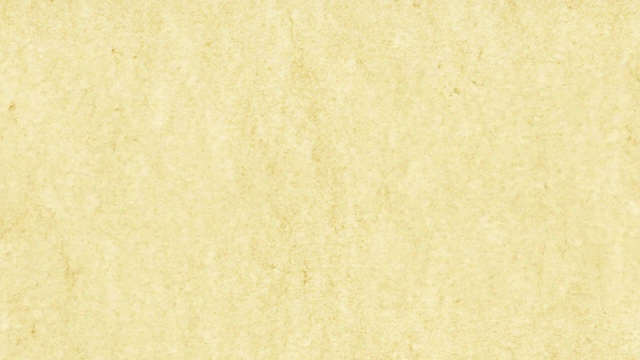 Hey, everyone, thanks for watching. To keep up to date on the newest videos from the channel, make sure to hit the subscribe button down below. I'll see you next time. In the meantime, keep pursuing history. Bye, Bye, Bye. Bye.